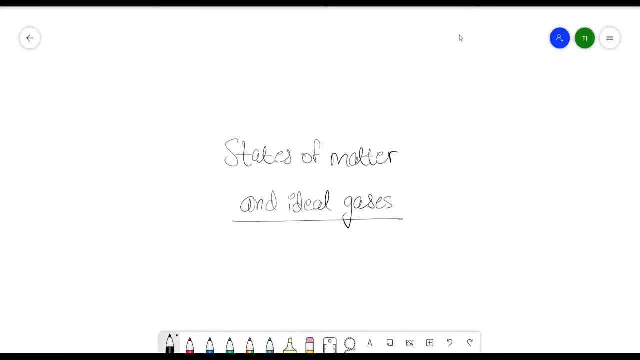 Hello everyone. today we'll be covering a very small lesson, which is states of matter and ideal gases from CIL or AS chemistry. This lesson is fairly simple. It's comprised of introduction, or basically a recap here- because you've done IGCAC, I'm assuming- of the three states of matter. 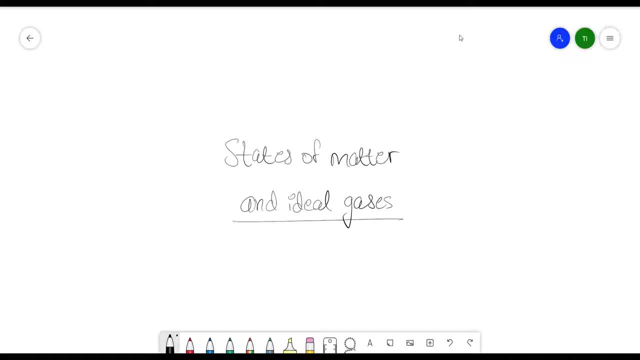 solids, liquids and gases and the different structures and their characteristics. and the new things in this lesson is the ideal class equation and the kinetic model of assumptions which these ideal gas equations are based off of, and simple volumetric conversions. lastly, some additional points that are important that are that don't really follow. they don't really fall. 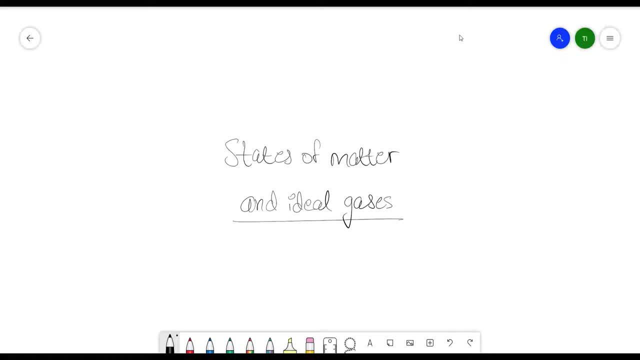 into any of the categories that we'll be learning today, so I guess they're miscellaneous anyway. let's moving on with the lesson. so, as you recall, there are three basic states of matter: a, and that is, solids, liquids and gases. well, excluding the, the plural form is just solid. 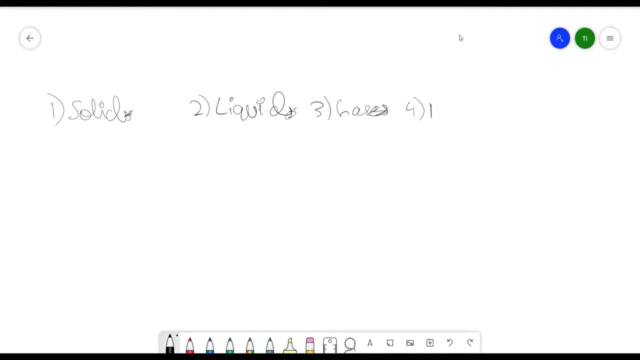 liquid and gas. if you do AL physics, then there's also a fourth state of matter called plasma, which you'll learn about more in the nuclear physics of a2. but since you're in chemistry, that isn't really within the syllabus, so we won't be learning about that or covering anything about that. 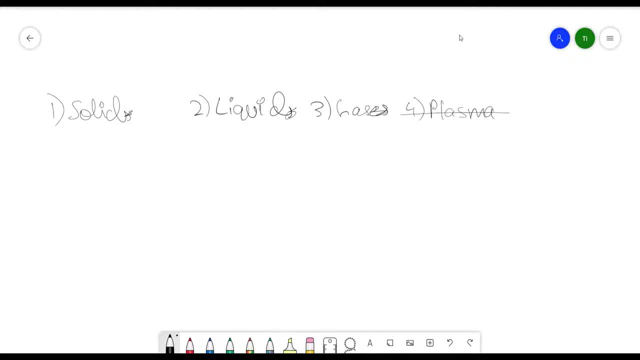 so, regarding solids, as you know that they have fixed mass. well, all of them have fixed mass, same thing. and solids have a fixed shape and volume. liquids do not have a fix shape because solids, Monster molecules, don't or may cells not be in a versus with such solids. 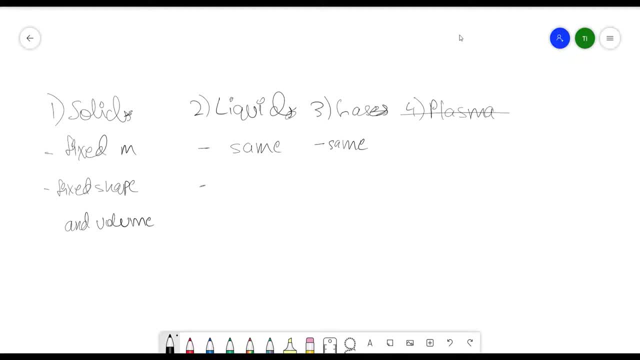 so fucking help market. okay, to just think about that, it's Agriculture home. Atomic Lemurs do not have a fixed shape, but the volume is fixed, whereas for gases they also have no fixed shape, but their volume is that of the container. they actually do have like fixed volumes as well, like there's a certain volume of gas. that's. 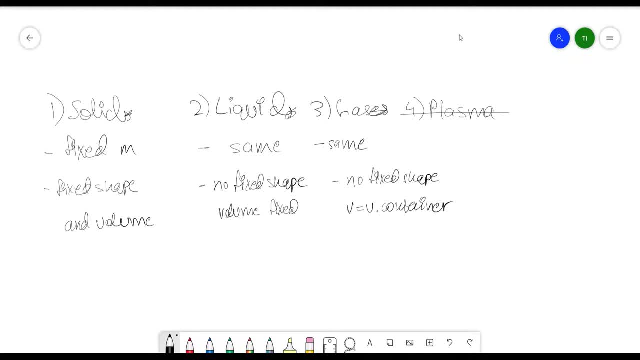 present within the container, but because the gases move about and have no forces of attraction between them, while most of them we just assume that it takes up the volume of the container. that's why we say it's what it does not have: a fixed volume. and regarding more about the particles of the objects in this, these 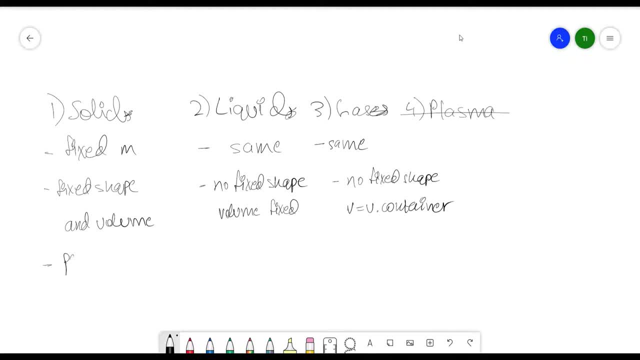 states and solids- the particle just vibrates or oscillates at fixed positions- and liquids, but the particles move around each other. and in gases the particles are well. they don't necessarily interact, they mainly just collide with each other, often influence the quality of life, size or magnitude, and the properties of these states are dependent on the molecule. 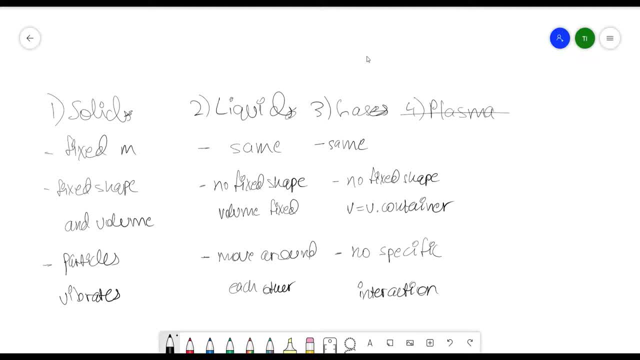 itself or the compound itself, for instance. I cannot generalize and say that solids have a high melting or boiling point, because there's solids that solid can't slow down, eliminates them onto the厲es. it can collate with other solids. so that's what obviously capable for estimated. 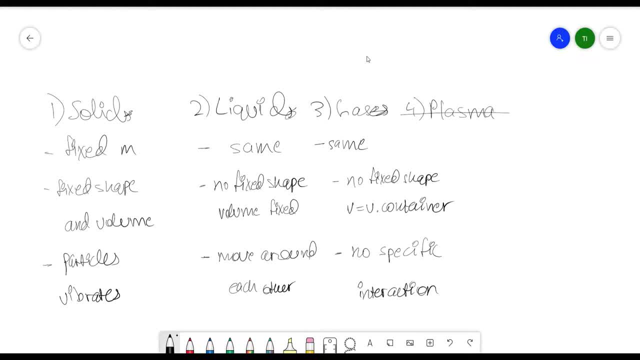 but its melting point is really high. i believe it's above 1500 degrees celsius, whereas iodine is also solid, but um, its melting point and boiling point is much, much lower, like in the 50s to 100 degrees celsius. so the properties depend on the compound itself. so there is an engine property. 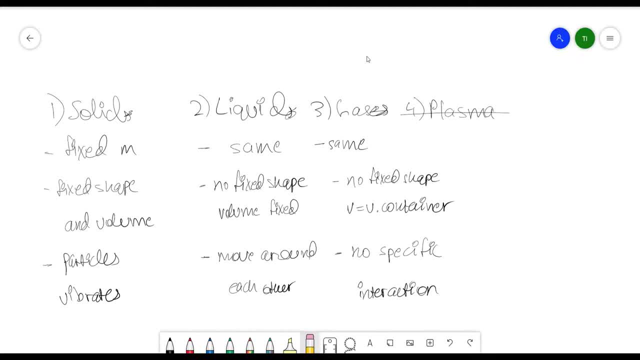 when it comes to that. so that is just a brief overview of, or brief recap of, what you learned in your igcse years. uh, they don't ask much about this, but it's best to keep it in mind, okay, uh, the next thing we'll move on to. uh, what we just covered is a recap of solid liquid and 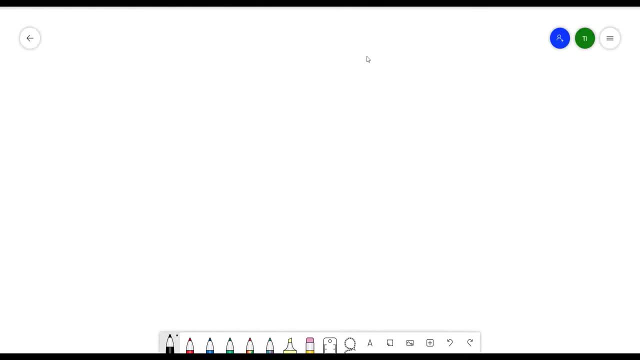 gases and their structures and characteristics. um, the next thing we'll move on to is also another recap and something that you've come across in the previous lessons: uh, when i talked about the chemical bonding between, uh, the different types of chemical bonding and the structures they form. so the different structures are in your syllabus, are the giant. 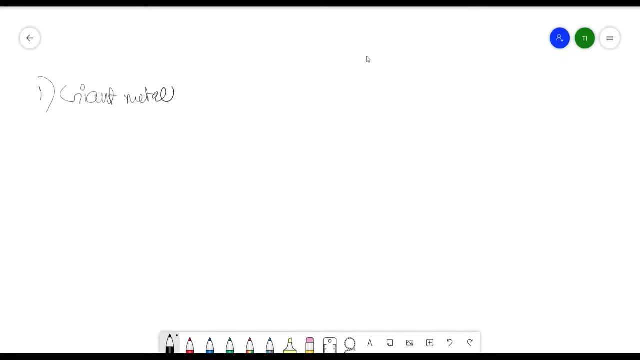 metallic lattice is formed. when, like metallic bonds, are formed metallic lattices, the properties are: you know what the metallic bond is, right, the you know how the lattice looks like. now we'll just talk about the characteristics. characteristics: if you do not know or remember what the shape of the lattice is, i suggest you. 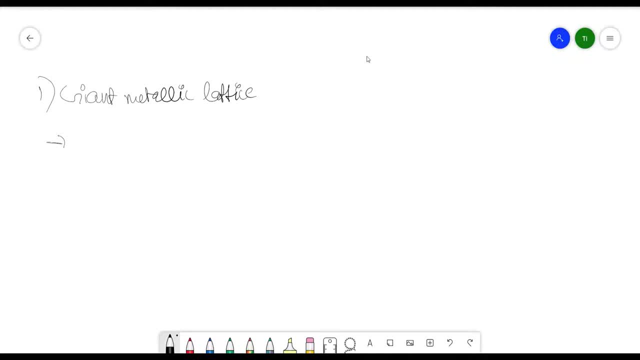 take a look at our previous videos. uh, so the characteristics are: layers can slide over each other and the- these are the most important characteristics. this is something that you should keep in mind always- that they're malleable, ductile and sonorous. and the last thing is that the electrons are delocalized. 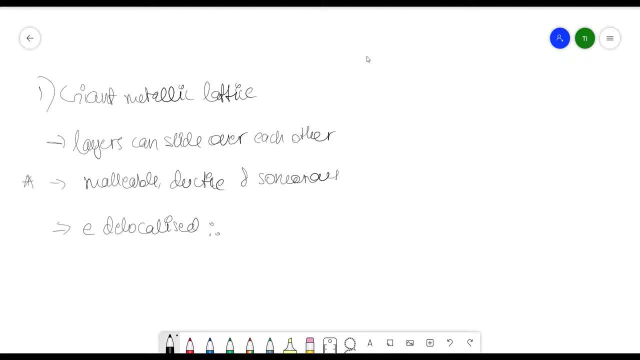 therefore, the giant metallic lattice can conduct electricity. so this is something that you have to keep in mind. yeah, now, these are the three characteristics that you have to keep in mind, where this is the most important one, so this is something that you must not forget. the next structure within your syllabus is alloys. 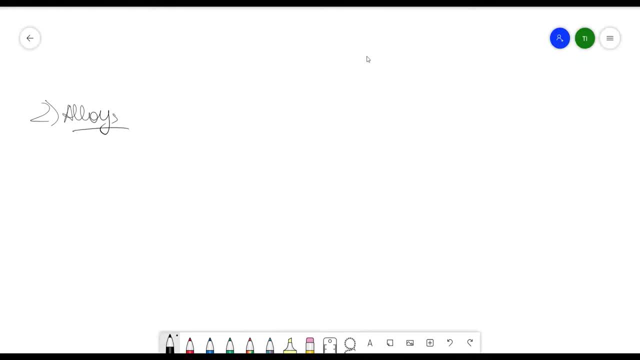 yeah, and what alloys are? basically, if you remember from the previous video, you know that alloys are the same thing, but if you remember from your igcc years, there's just a mixture. of metals can be of different person, different percentages and the different cationic size, like the cations, because they're different metals, so the cationic 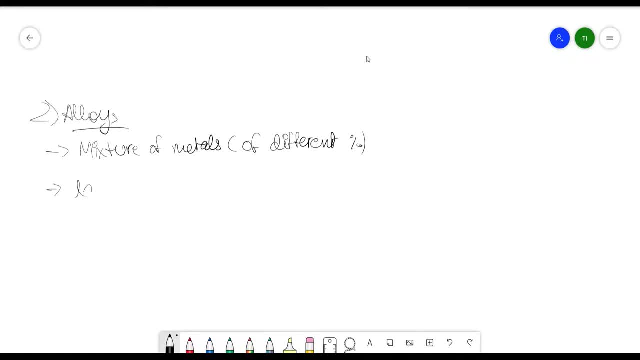 size is different because the cationic size is different. uh, the layers cannot slide over each other as efficiently and in most cases, alloys are stronger than pure metal. for example, the alloy stainless steel is stronger than iron. yeah, then we have simple molecular structures, and these are formed primarily by molecules that have covalent bonding between them. their 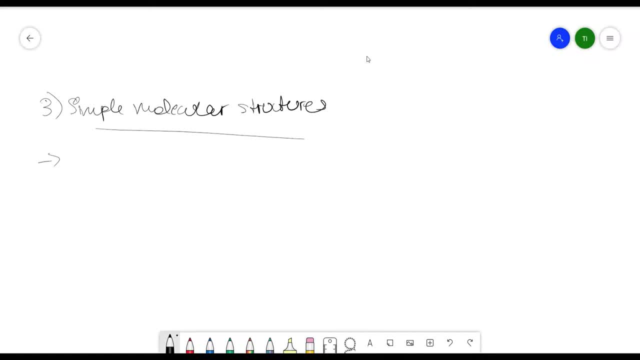 characteristics are? they form them. they mainly form liquids or gases, but if they do form solids that have weak- sorry, low- MP and PP- magic once, and boiling points and the IMF are easily broken when heated. so therefore, like this. this is the reason for this. the next type of structure is: 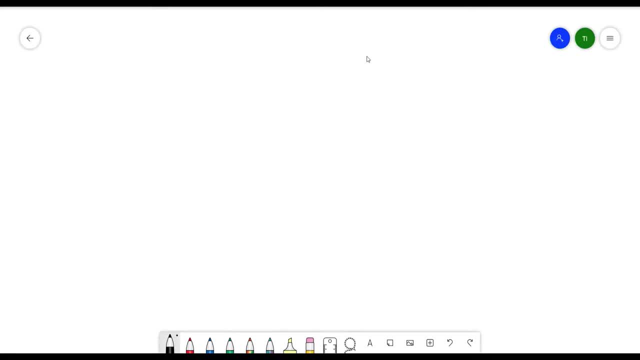 Giants molecular. I remember this is the fourth or fifth, I suppose the fourth giant molecular, and then later they're. they're mostly not conductors, except for graphite, uh, but they have high MP generally- not always, and uh, that's pretty much it, I believe, and the layers can slide over each other in some cases. no, these 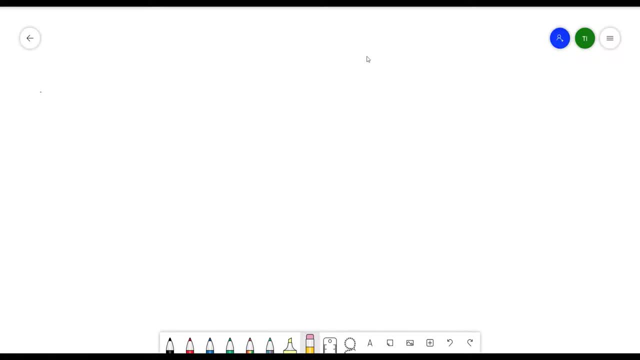 are also not generalized, so they don't have specific trends, but generally they have high melting points and boiling points. so some examples of uh, giant molecular structures they need to know about are graphite, graphite diamond, diamond and silicon dioxide- sorry, not yeah. silicon dioxide, which is basically silica. yeah and uh, you must know that this has high MP and BP. 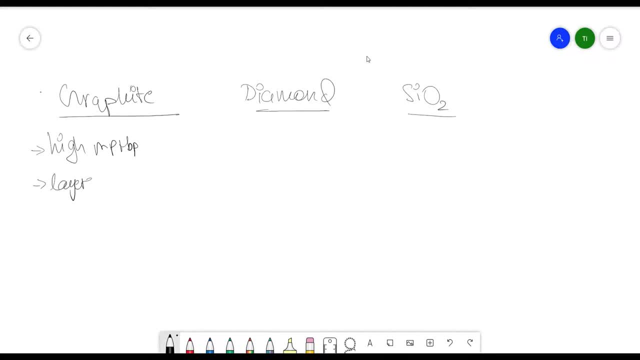 layers can slide. therefore uh can be used as lubricants and each carbon atom is one, two, three other carbon atoms, so they have like delocalized electrons and therefore are electrical conductors. sorry, conductors. yeah, these also have high melting point plus boiling point. they're non-conductors. 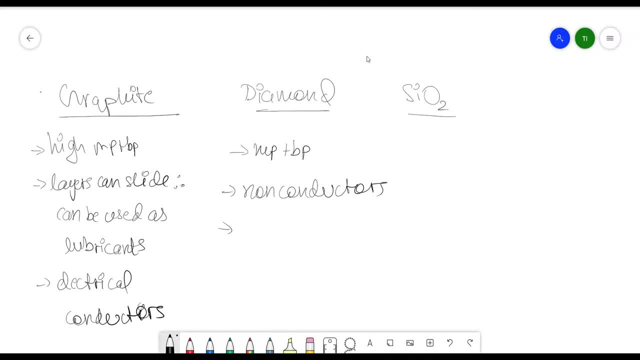 and since you have done uh molecule shapes, now you should know what the tetrahedral structure is, because each carbon atom is bonded to four others. uh, it has an spc, hybridization and therefore tetrahedral structure, and that's pretty much it. and silicon dioxide is similar to that of diamond. 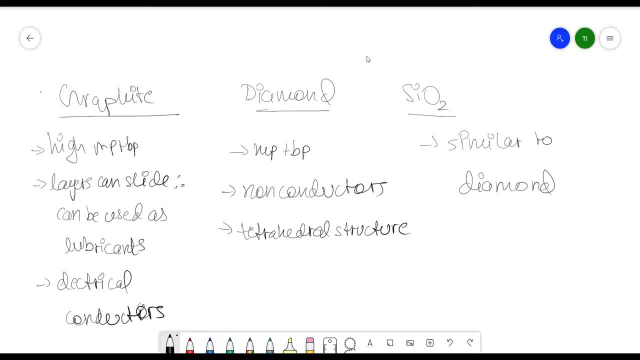 yeah and uh. for those of you do not know, silicon bonds like four other atoms and this is how it bonds to it. so there's one silicon, uh, two atoms and this is how it bonds to it. so there's one silicon, Si, Si, Si and Si right, and in between each of these there's an oxygen atom. 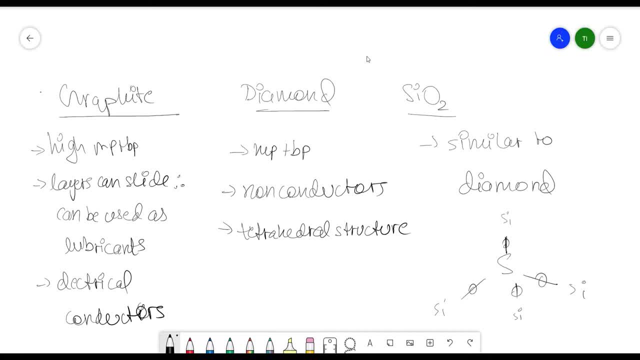 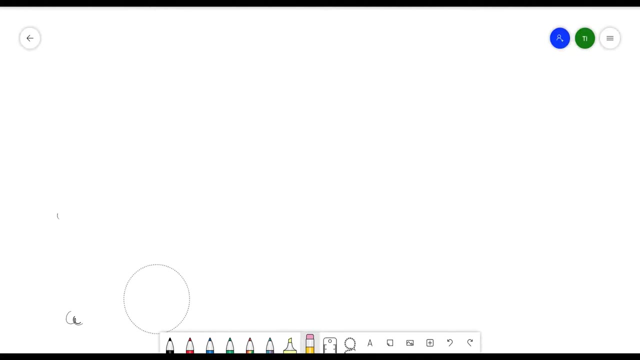 that's what the structure of silicon dioxide looks like. if you want a more visual representation of this, I suggest you check out images in Google. now there are two more types of carbon allotropes that are within our syllabus, and that is C60 fullerene and, yeah, C60 buckminster- I believe it's buckminster. I saw buckminster. 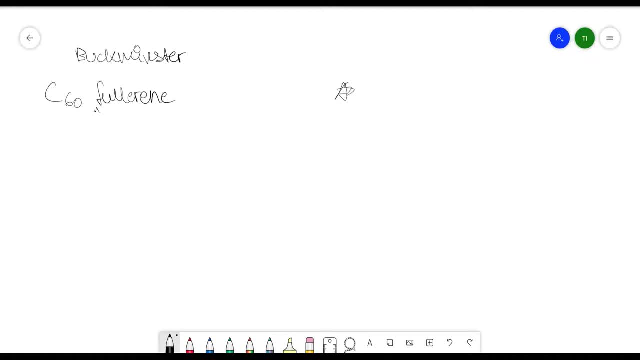 fullerene, and there was another one anyway about this. so it has 60 carbon atoms, yeah, and they have simple molecular structure and therefore have relatively lower melting and boiling points. okay, and one more thing about them is that they can, and I repeat, can- conduct electricity. they can conduct. 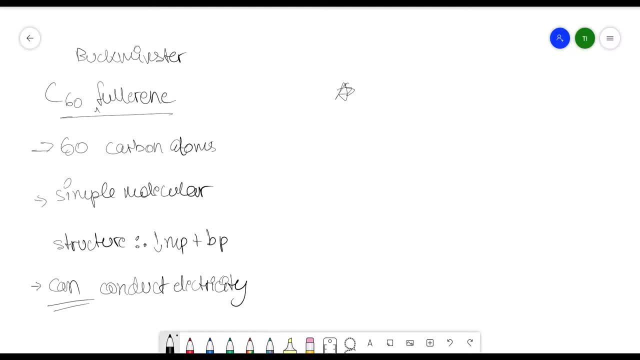 it's not always that they will conduct, but they can conduct electricity anyway. the other one is is something known as graphene, and these are much better conductors electricity. yeah, much better conductors of electricity. uh, and in the past syllabus. not in the past syllabus, even in the current. 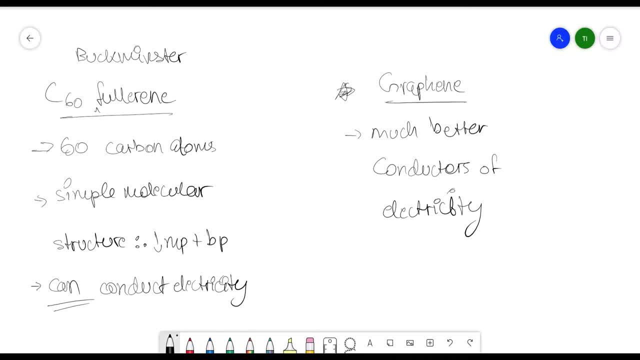 syllabus, but they don't ask it as much. but if you do, uh, practice a2 papers from before 2016, you'll see that the paper fours have something called nanotubes. so whenever a nanotube comes, what you have to understand is that its size is. 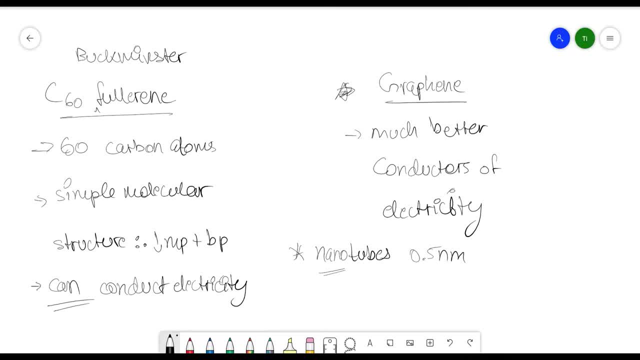 very small, so approximately 0.5 nanometers. that is the size of the diameter of the tubes, and that is basically what a nanotube is. that is formed, uh, that is formed with carbon. now, that is all about the carbon allotropes within your syllabus. 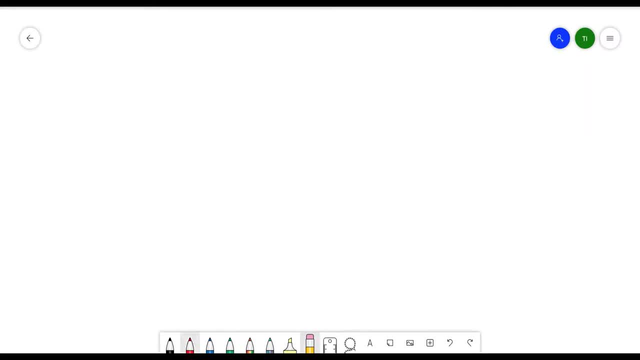 i just briefly went over it, uh, because these are things that you learned in igc sc. i didn't go much into depth. anyway. the last part of this lesson is the ideal gases and the ideal gas equation. now, before we go into ideal gas equation, what you have to know is the kinetic model of assumptions. 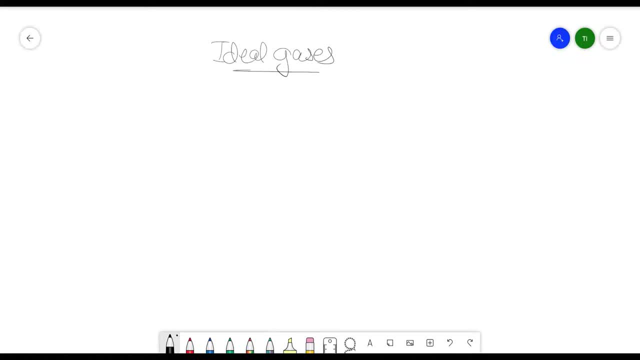 that the ideal gas equation is based off. uh, if you did a2 physics or if you did sat physics, then you'll know, you'll be very familiar with this lesson, because it is from thermodynamics. uh, in chemistry we don't really go into the derivation of the ideal gas equation, so you just have to accept it at phase. 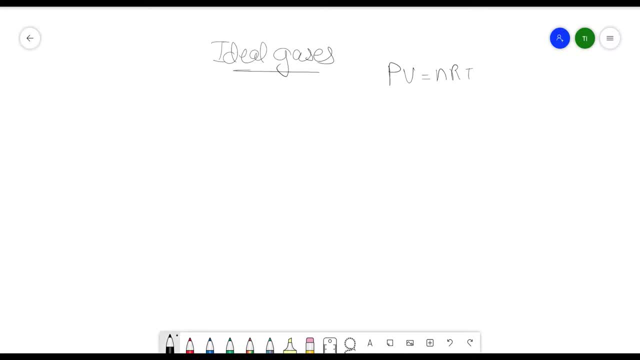 at phase value, and this is the formula: pv is equal to nrt. where pv is equal to nrt, and this is the formula: pv is equal to nrt where pv is equal to nrt. where pv is equal to nrt, p is equal to the pressure in pascals. 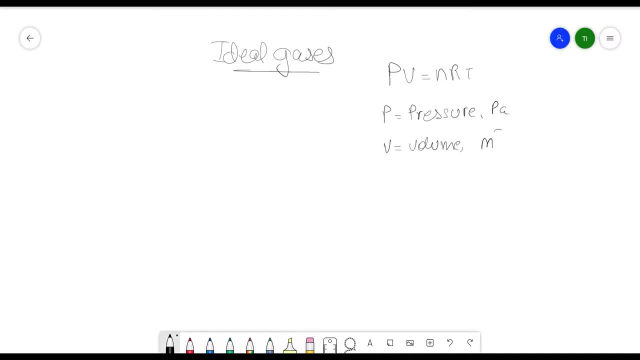 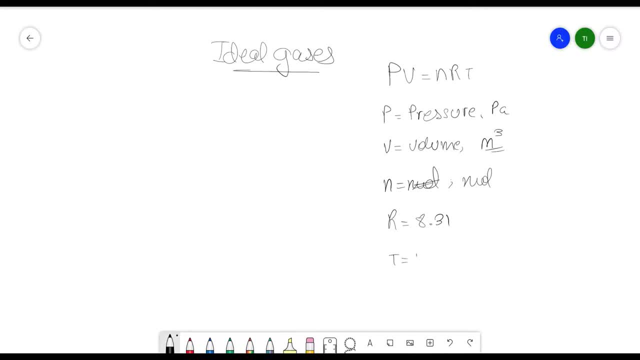 constant. ideal gas equation: constant and t is the thermodynamic temperature, which is in kelvins. now some basic conversions that you need to know is: for t in degrees celsius to t in kelvin, you have to add to t and degrees celsius you have to add 273. 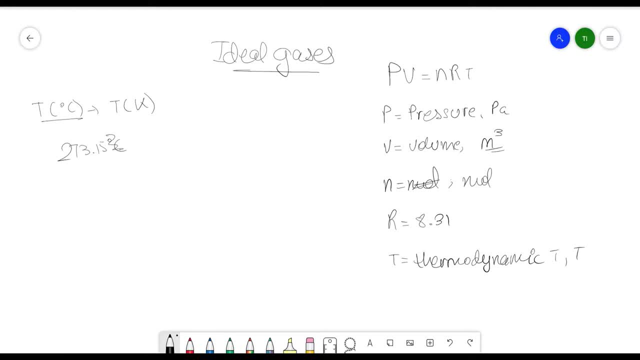 273.15- sorry, 273.15, to convert it to t in kelvins. uh, in your syllabus it's okay if you convert it, uh, if you add only 273, but this is more accurate, so i prefer doing it with 273.15. 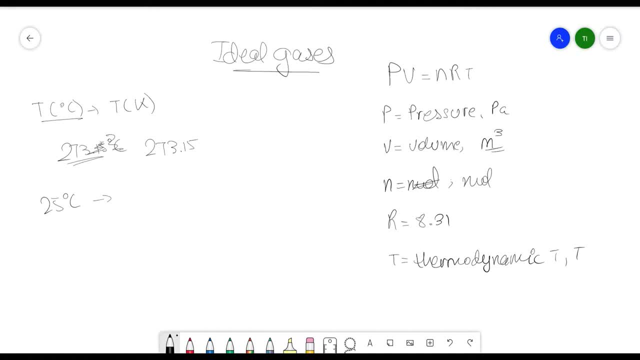 so, for instance, um 25 degrees celsius. how would you convert it to kelvins? the answer would be 25 plus 273.15, which would give you 298.15 kelvins, and it's the same way around. if you want to sub. 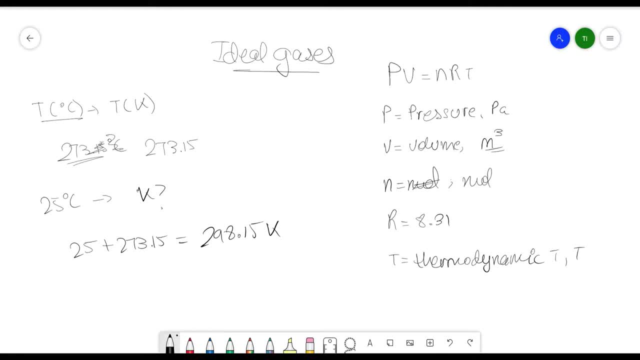 if you want to convert from kelvins to degrees celsius, all you have to do is subtract it with 273.15, yeah, and you'd get the thermodynamic temperature. whenever they mention thermodynamic temperature, then you have to give the temperature in the unit of kelvins. that's an important conversion. another important conversion. 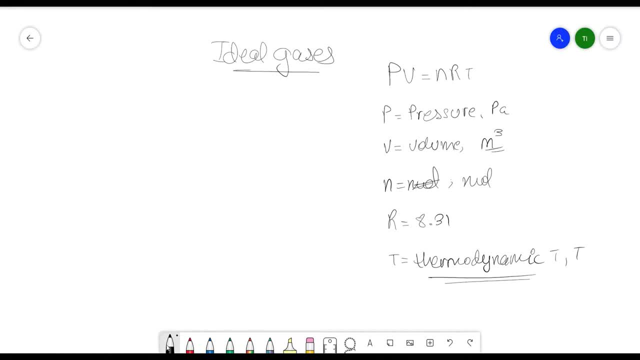 is conversion, like the volumetric conversion. so because you have to use meter cube in this one, you have to know how to convert from cm cube to meter cube and from dm cube to meter cube. so to convert from cm cube to meter cube, uh, you remember that to convert from cm to m you have to. 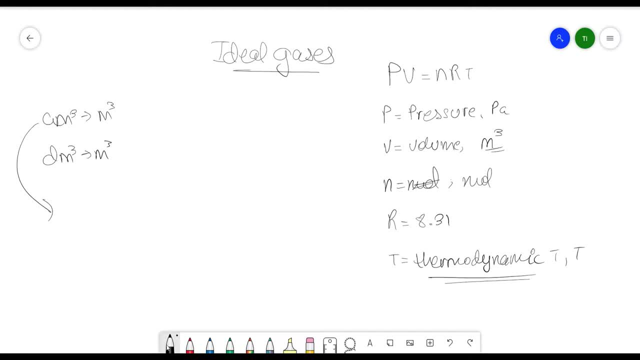 divide by 100. so if you want to convert one centimeter to meters, you have to divide one. divide by 100 and you get 0.01 meters right now. similarly, if you want to convert a centimeter cube to meter cube, all you have to do is divide it. divide divided by 100 cube. so let's say: 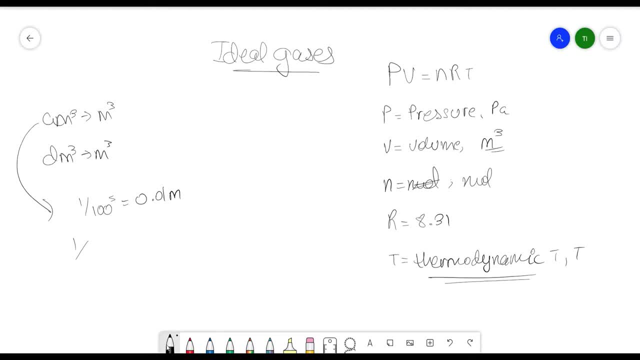 you want to divide 100 centimeter cube. the centimeter has been cubed right, so its conversions would be cubed as well. so it'd be divided by 100 cube, which is, i believe, really small value. one into 10 to the power, minus six meter cube. yeah, to convert dm cube to meter cube, all you have to do is 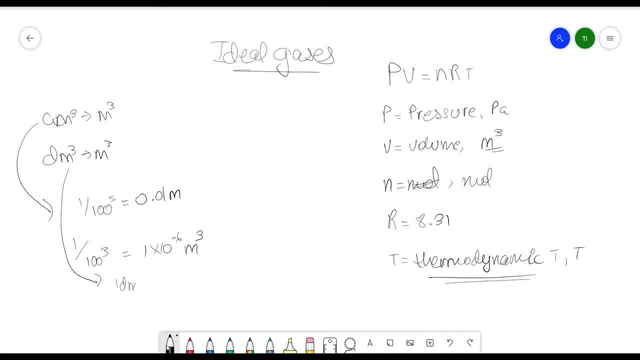 divide by one thousand. so, uh, let's say you have one dm cube. to convert it to meters, meter cube, you have to divide by one thousand and you'd get one into ten to the power, minus three meter cube. uh, for dm cube to meter cube, i prefer doing it like in steps rather than like this, which is first. 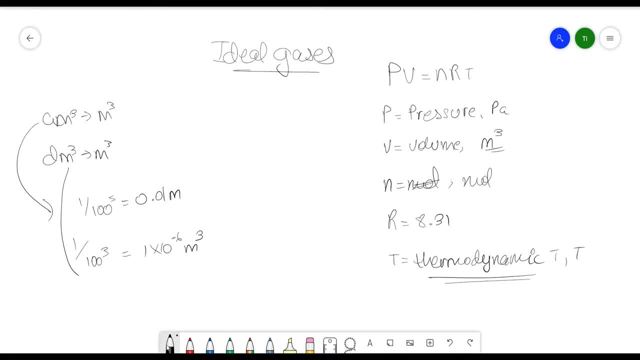 converting it to centimeter cubes. so dm cube to centimeter cube is into one thousand. so that would be, uh, one into one thousand, which would be one thousand cm cube, and divide this by one hundred cube, so one thousand divided by 100 cube, which would give you the same answer one into 10, to the. 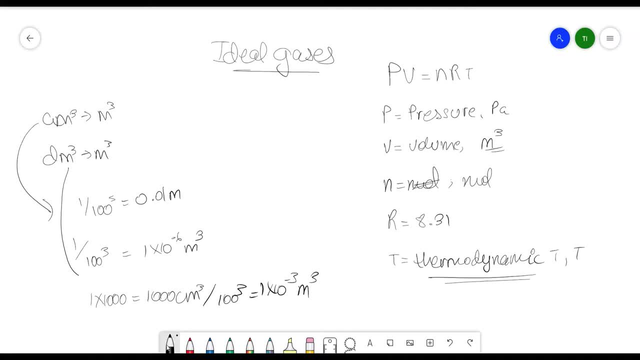 power minus three meter cube. the reason why i do this is because it helps me remember the conversion of dm cube to centimeter cube, which is very important in stoichiometric calculations. now that this is also an important conversion that you need to know. okay, now let's get into the 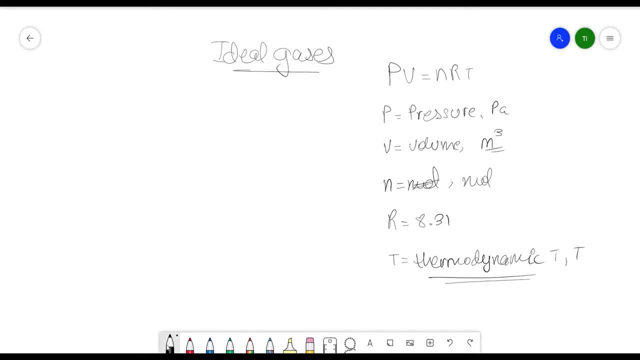 statements, or this is basically the kinetic theory, uh, based on which the ideal gas equation is formed. this is the ideal gas equation, okay, and it basically is like the simplest way to remember it. okay, how did this turn into a pentagon? i don't understand. okay, it simply is like the base, the best way to remember. 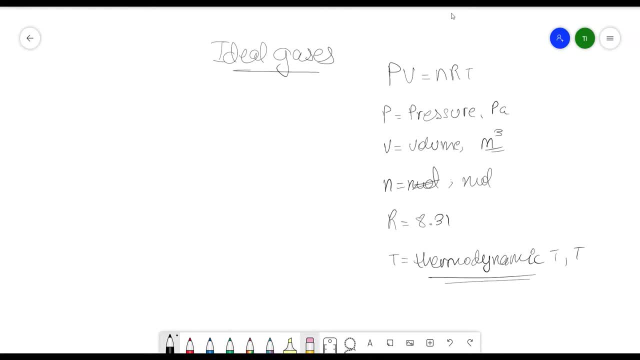 it because you don't have to go much into an understanding of what it is. wait, let me just erase this from the side so i'd have more space. the best way to remember it is by ravid. i'll also explain on the side so that you understand, like what each of the statements mean. 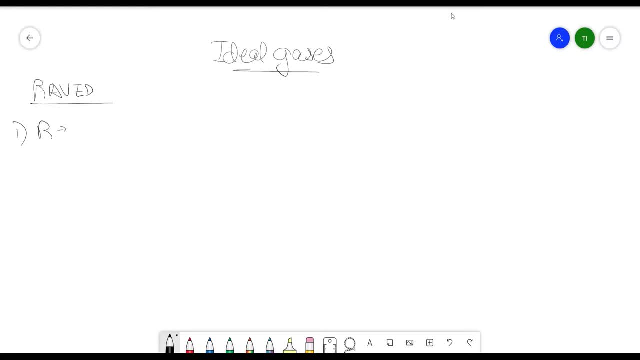 so ravid. the first part is r, which states random collisions, so random and rapid motion of molecules. okay, random and rapid motion of molecules, which the first word is r and that's why it's r. uh, sorry, the first letter is r and that's why it's r. and what random and rapid motion of molecules. 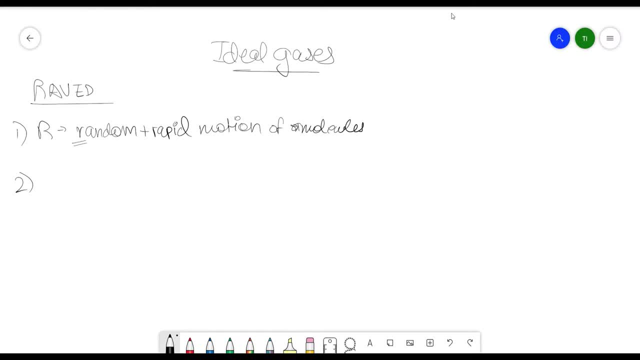 means is that the motion is completely randomized, it does not have any trends. uh, the second assumption is that a so attractive forces between molecules are negligible, such as imfs, so let's say normally: uh, an atom such as diatomic atom, diatomic molecule such as bromine. 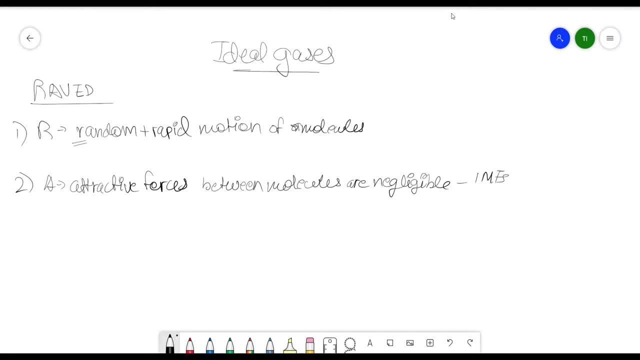 uh to. to consider it as an ideal gas, we have to ignore the intermolecular forces that are present between the Roman molecule. the third is V. so volume of gas: negligible. negligible relative to volume of container. so let's say the volume of gas is what? around one meter cube and the 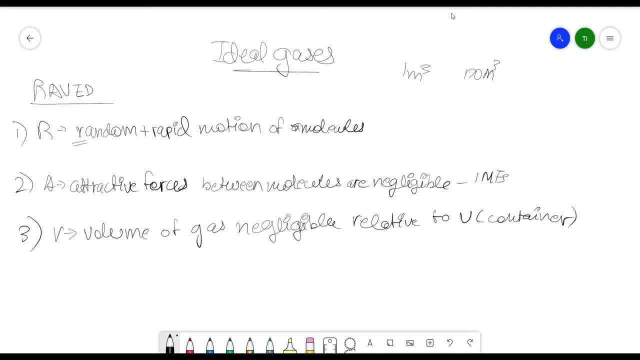 volume of the container is 100 meter cube. that's a lot, but just as an example, please accept this. so, even though the gas is one meter cube, how did this turn into a triangle? I do not understand. so, since the, since the, even though the molecule, the volume of the gas is one hand, one meter cube, it occupies. 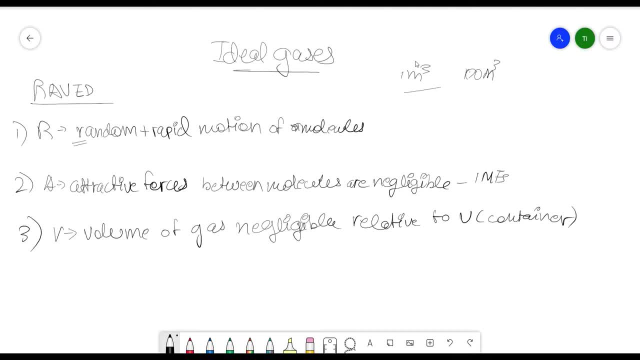 volume of gas negligible- negligible relative to volume of gas. negligible relative to volume of gas is one meter cube. it occupies the container that it is filled like. that fills right and therefore we assume that the volume of this gas is negligible in comparison to the volume of the container which it occupies. that is basically what the third statement 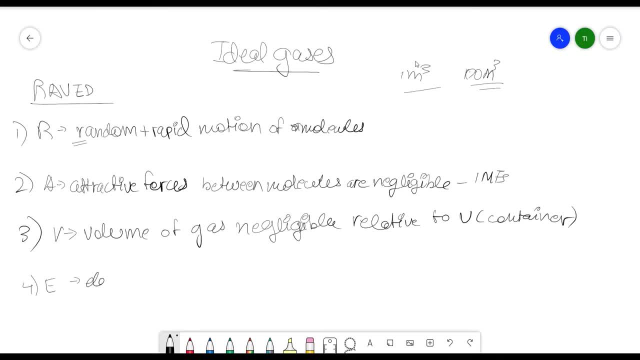 the third statement is. the fourth one is E, which means elastic collisions. for those of you who have done physics, this must be a very familiar term. elastic collisions basically means that there is no loss of velocity, momentum or kinetic energy in between the collisions. and the fifth statement is regarding 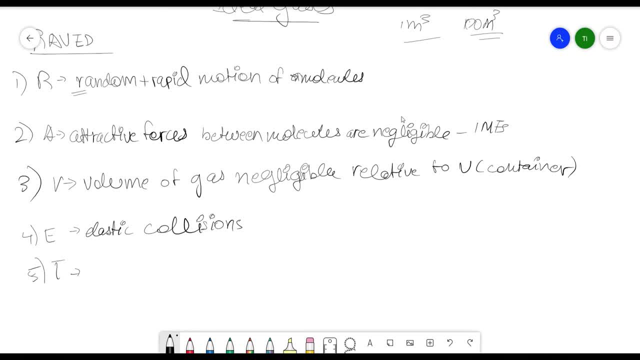 time. so time of collision is negligible in comparison to time between collisions. so what it basically means is that when two molecules, two atoms, collide, okay, the time like that this collision happens for is negligible in comparison to the time between the collision, so when they will collide again. so let's say the molecules are here, right, sorry, the atoms. 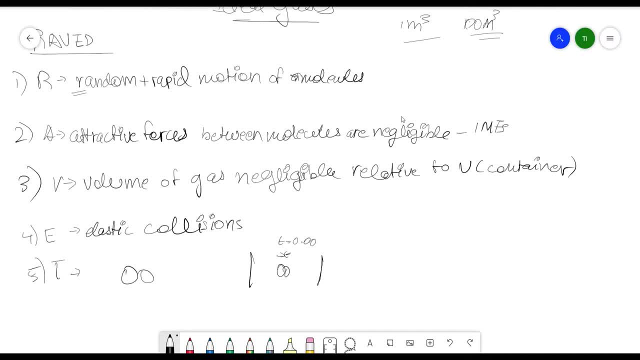 are here, they collide and let's say this: T is 0.001 seconds, okay, and for them to collide again, you would see them collide again again after approximately two seconds, and therefore this time is negligible in comparison to this. that's basically what the fifth statement means. now you don't really have to go into an 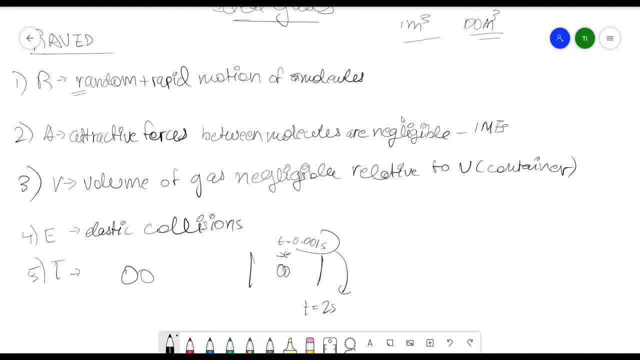 understanding of what each of these statements mean. you just have to by heart these statements and be able to recall them and use them whenever asked for. I hope that makes sense. the base, the best way to remember it, is wrapped. okay, now let's do a small question. I'll provide, I'll give it the 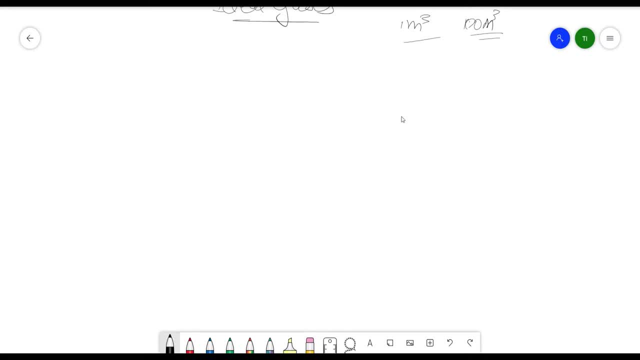 values and you just have to do the calculations after pausing the video. so the question is the volume of carbon dioxide at temperature of 298 kelvins and pressure of 100 kilopascals, and the mass of carbon dioxide given is 2.2 grams. pause. 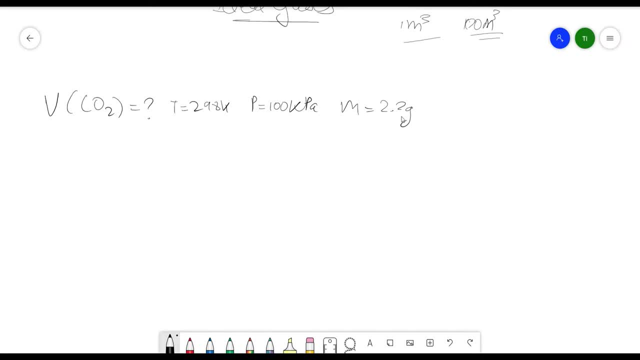 the video and have an attempt yourself. anyway, the way I do this in steps is first convert everything to SI, the units required. so you see that the pressure given is in kilopascals. you have to convert it to pascals itself. so kilopascals of pascals is 100 times 1000, which is 100 times 1000, which is 100 into. 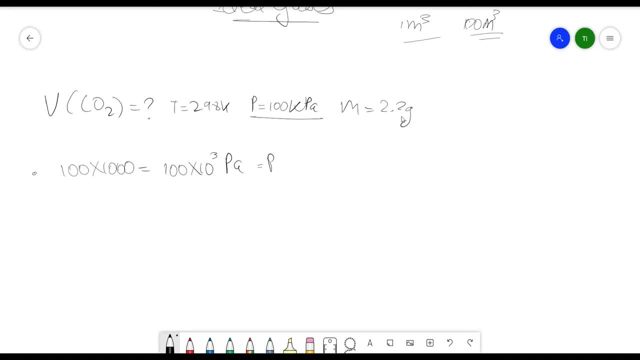 10 to the power 3 pascals and this is the pressure and they've given you the mass of carbon dioxide. but in the equation PV is equal to an RT. you need the most. how would you get the most? and the molds would be m by MR. 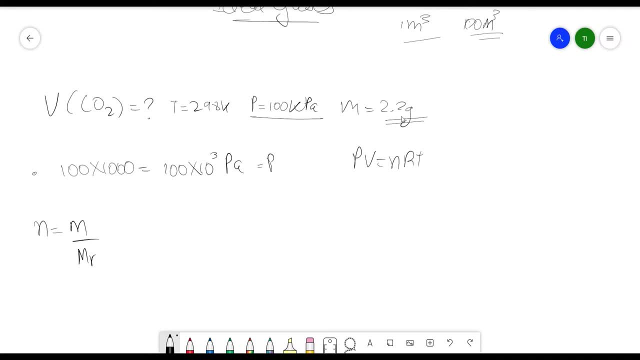 understand that I haven't thought psychometry yet for the is level, but this is something that you turn IDC s and therefore should remember from your IGC- see yours. so i'm by a more. so should be 2.2 divided by the Mar of this. so it will be. 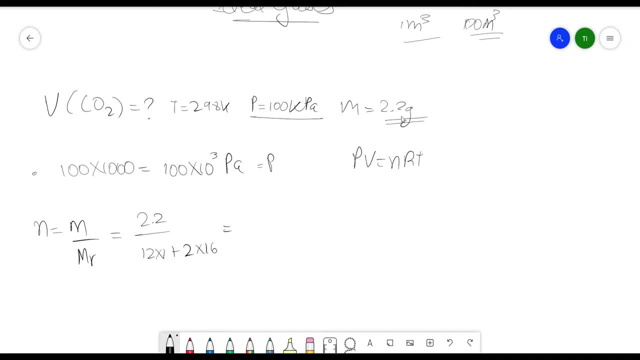 12 into one plus 2 into 16.. So that would be 2.2 divided by 12 plus 2 into 16.. That would be 0.05 molts, right? So how would you find the volume of carbon dioxide? So the volume would be: 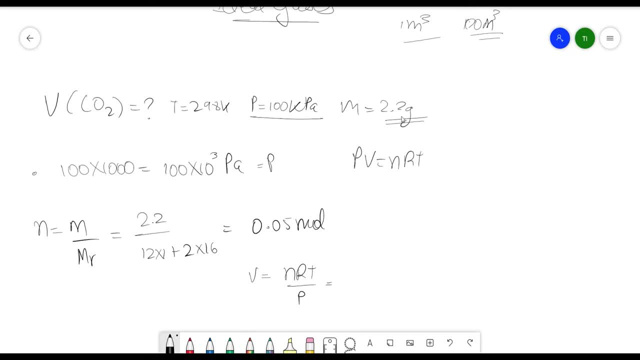 nRT by p, So the n is 0.05, R is a constant 8.31, and T is given to 98 kelvins, divided by the pressure, 100 into 10, to the power 3.. And the volume you would get is well, let me just do the. 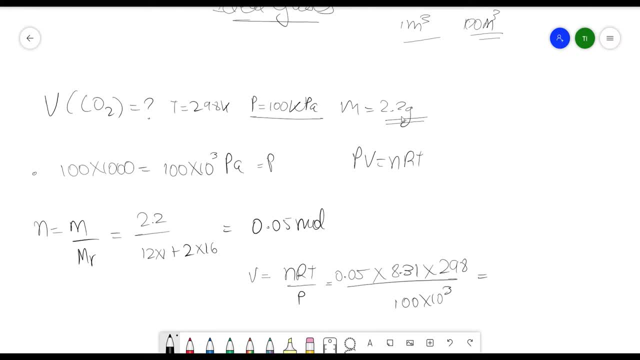 calculation on the calculator: 0.31 into 298 divided by 100 into the power 3.. So the volume you would get is 1.24 into 10 to the power minus 3 meter cube right. And if you want to convert, 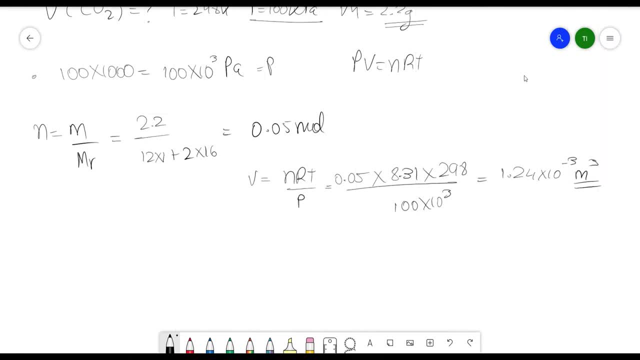 this to, let's say, dm cubed. how would you convert it? To convert it into dm cubed, you just have to multiply this value into 1,000. And to convert it into meters cubed- sorry, centimeter cubed- you just have to do it into 100 cubed. I hope you understood. Now let's take 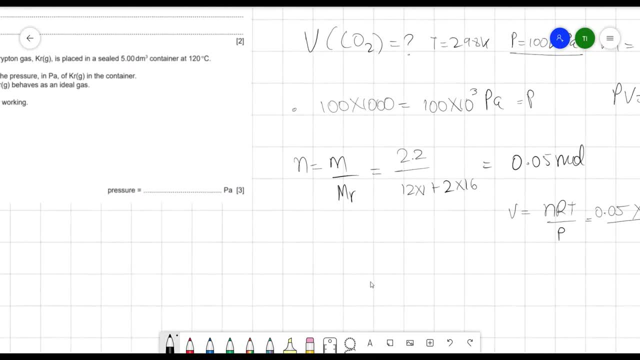 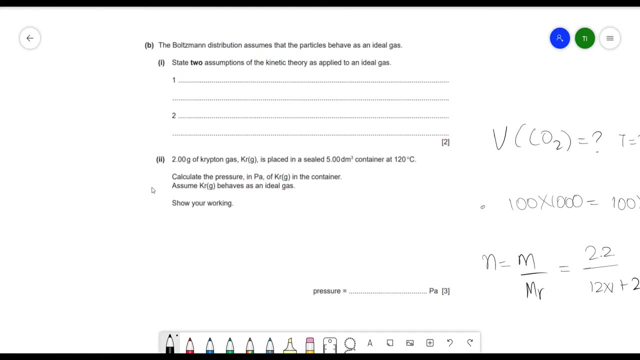 an example from a past paper that is very recent paper as well. I believe it's February, March 21.. So, as you can see, the questions are very similar to what I've taught. So the first question in that: the Boltzmann distribution, which is something you're going to learn in the rates. 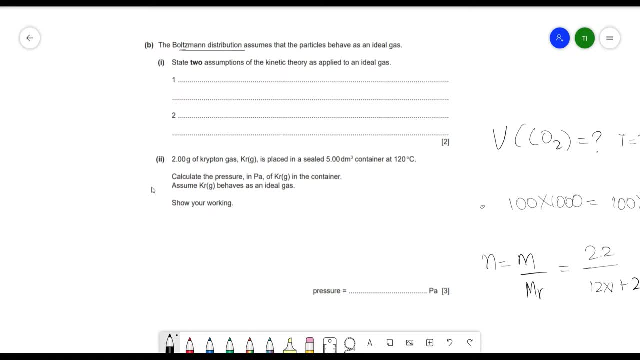 part. but we don't need that. Well, we don't need that knowledge right now. assumes that particles behave as an ideal gas. right? So state two assumptions of the kinetic theory applied to an ideal gas. So any from these five, any two, So the easiest ones are E, so elastic collisions. 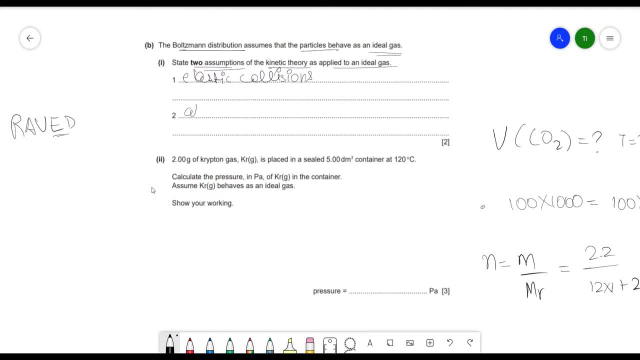 And another would be attractive forces. Attractive forces such as IMFs between gas molecules are negligible, And that's easy. two marks for just remembering this thing. okay Now, two grams of particular mass and gas which is placed in a sealed container of five DM cube. So that's the mass and that is the. 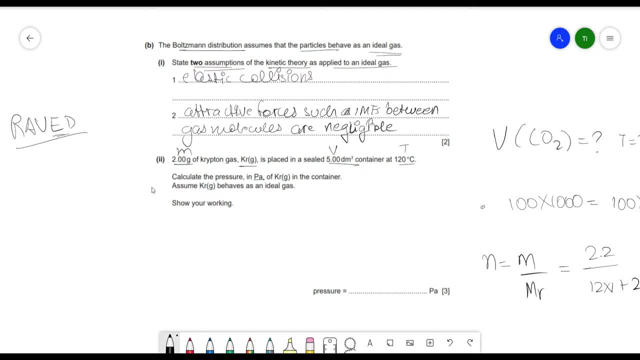 temperature right. Calculate the pressure in pascals of krypton in the container. Assume that krypton behaves as an ideal gas. So because it behaves as an ideal gas, you will have to use the equation. PV is equal to an RT. The value of R is given in your data booklet, so you don't have to. 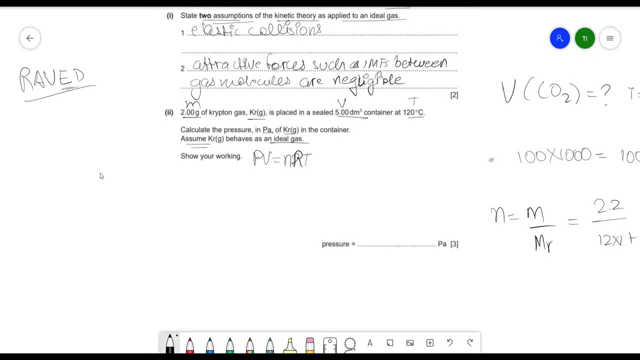 worry much about remembering it. So let's first convert everything into the units required, So V. so to convert DM cube into meter cube, five into 1000 is five into 10 to the power three meter cube. No, sorry, DM cube to meter cube, right, So I made a mistake, sorry. 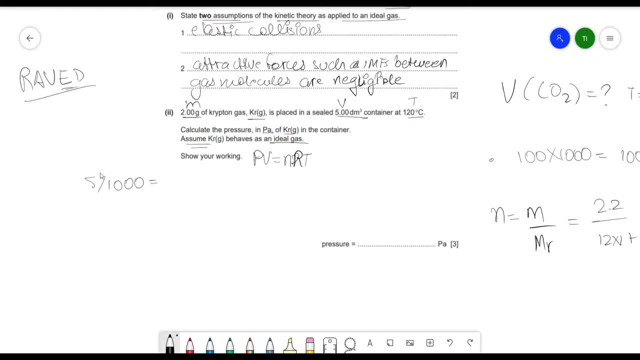 To convert DM cube to meter cube it has to be five. divide by 1000 is equal to five into 10, to the power minus three meter cube right. To convert temperature into Kelvin's it has to be in thermodynamic temperature. you have to add by 273.1. 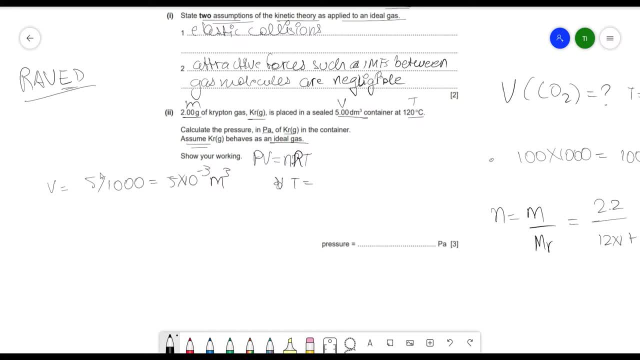 so 120 plus 273.15, that's 393.15. now you have temperature, you have volume, you have r, you need n. how would you get n? this is the same way as we did in the previous example. question n is equal to m by mr, and this is krypton, so it's a monoatomic gas. so the ar of krypton is something that you 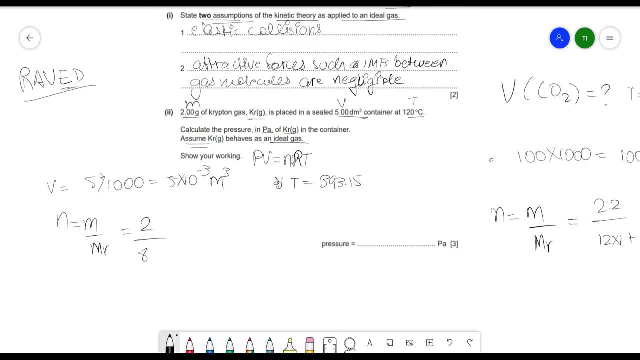 can get directly from a data booklet. so that is 2 divided by 83.8, if i recall correctly. so 2 divided by 83.8, which is at 0.0239 moles. in the calculator i got a much larger value. and when you're doing 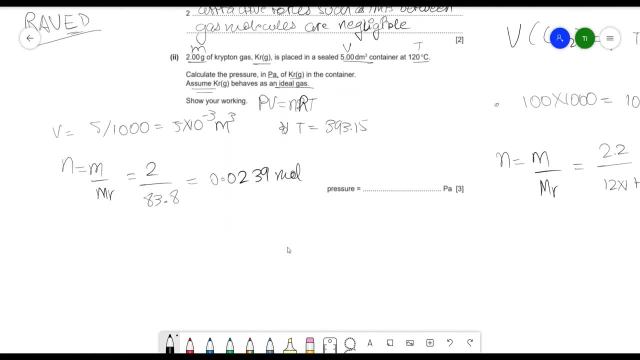 calculations do not run until you get the final answer, so i'm just going to use the whole value in my calculator. but in my workbook i'm going to use the whole value of the calculator, so i'm going to show that i'm using a rounded value anyway. so you have to make p the subject of the equation. 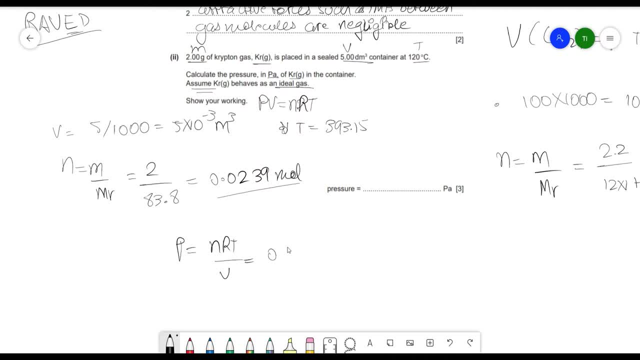 and rt by v, and therefore it would be 0.0239 into 8.31, into 393.15, the whole thing divided by the volume that we got, 500 minus 3, so which would give me 8.31 into 393.15 divided by 5 minus 3. 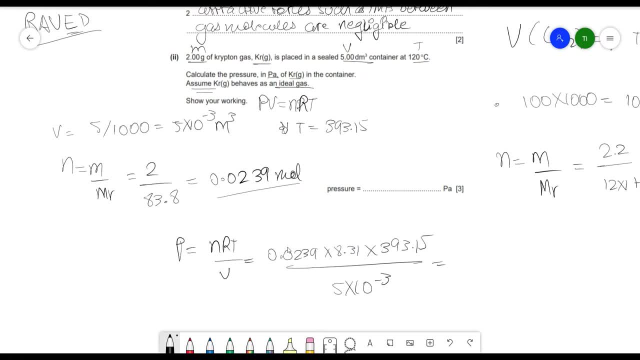 which would give me 15595 pascals. now you take a look at the values given, you see that there's three significant figures here, three significant, three significant. well, you can't really tell the significant figures of this. so, because majority of the values are given in three significant, 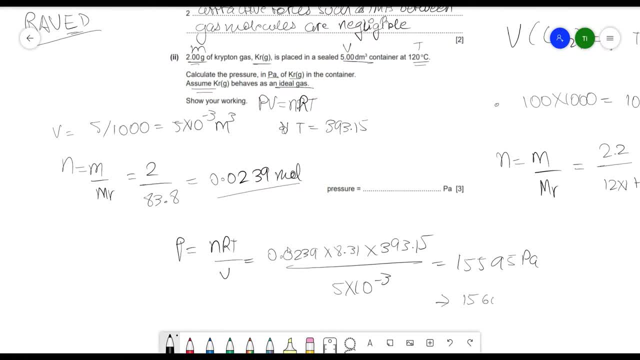 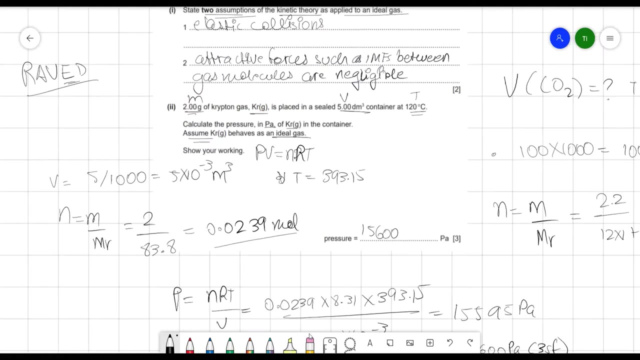 figures. you have to round this through csf, so 15600 pascals 3sf. now, yes, you got the right answer given in the answer space provided. otherwise they will not give you the last mark. so that is easy. uh, five marks in paper two. yeah, that is it for ideal gases. now some miscellaneous facts that you need. to know about the ideal gases. so these are some important miscellaneous and these i've gotten from solving doubts in past papers. now, the gas that behaves most like an ideal gas is helium, and that's because it's monoatomic and it has almost negligible intermolecular forces, because it does not have any other forces than 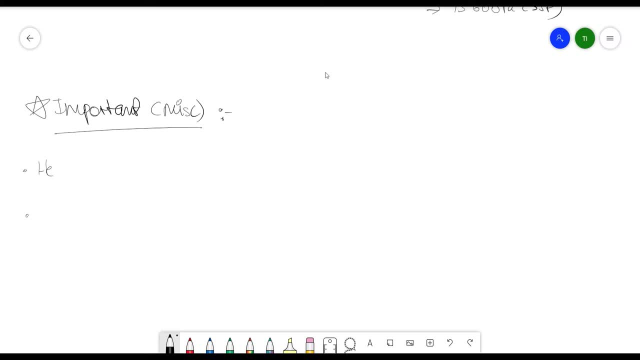 van der waals and only has two electrons, so the strength of van der waals attraction is very weak. okay, now another. okay, uh, sorry about that anyway. another, uh important fact is hcl, and it deviates to ideal gas behavior to ideal gas behavior. nh3 does not show. 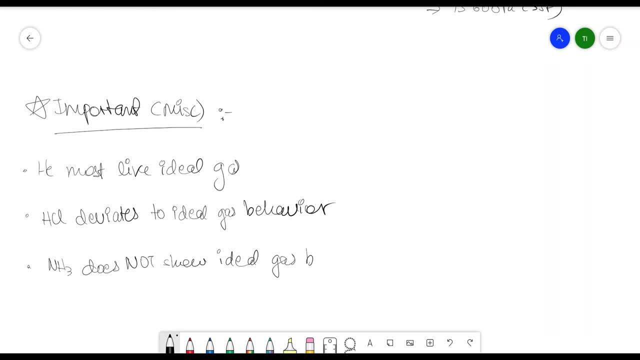 ideal gas behavior, and the reason why that is is because nh3 has, as you can see, h, h and h has one pair of electrons and because then it's a highly electronegative molecule, it has partial charges and hydrogen molecule. hydrogen bonds can form between the nrc molecules and that's why the intermolecular 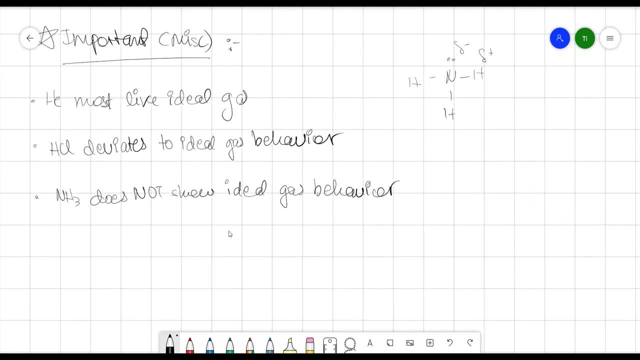 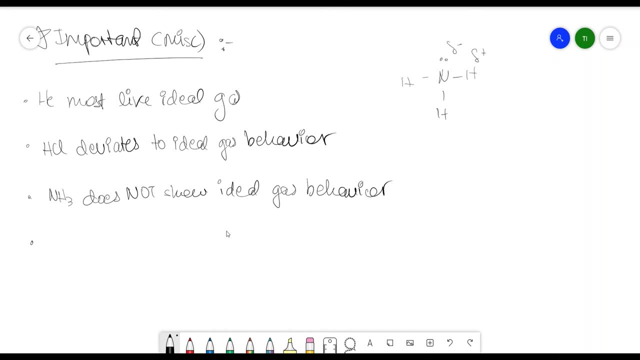 forces are not negligible, so it behaves- it does not behave like an ideal gas and um ideal gas equation- ideal gas equation- ige is best- is followed at low uh low pressure and high temperature, and this is based off of boyle's law, where pressure is invertedly proportional to inversely proportional to volume, so the lower the pressure, the higher the volume and therefore the particles are not as closely packed, so intermolecular forces are more negligible. and at higher pressures volume is directly proportional to temperature and that's why- sorry, at higher temperatures the volume is directly proportional to the volume and that's why intermolecular forces are more negligible. i hope that makes sense.